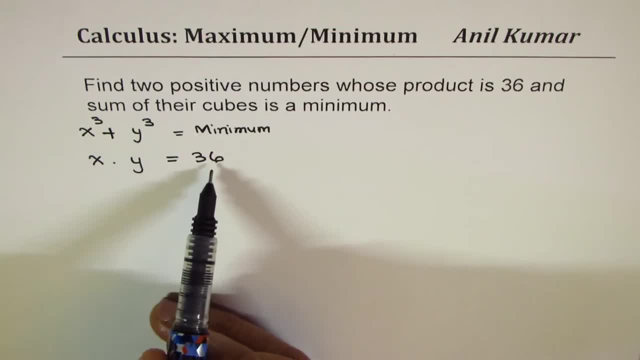 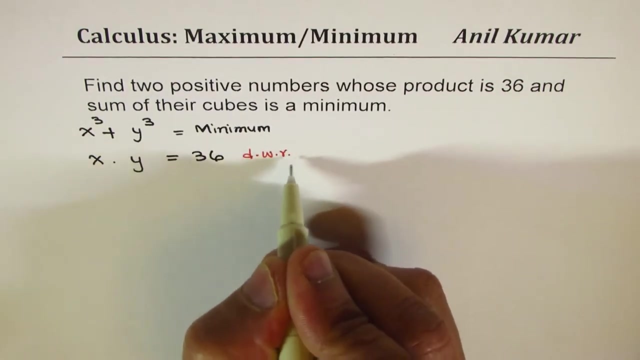 me relate dx, dy from equation number 2 here. So we have: x times y equals to 36.. So if I differentiate this equation with respect to x, that means I will differentiate this equation with respect to x. then what will I get? Both sides. So we will apply the product. 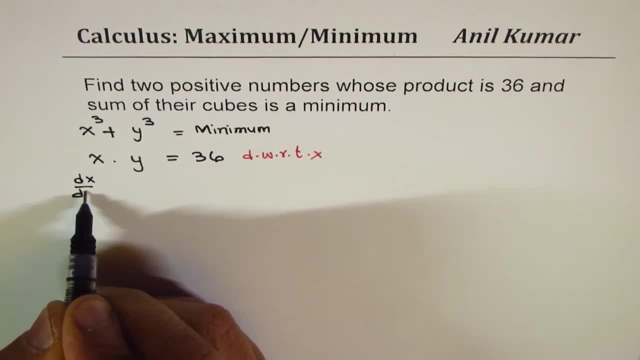 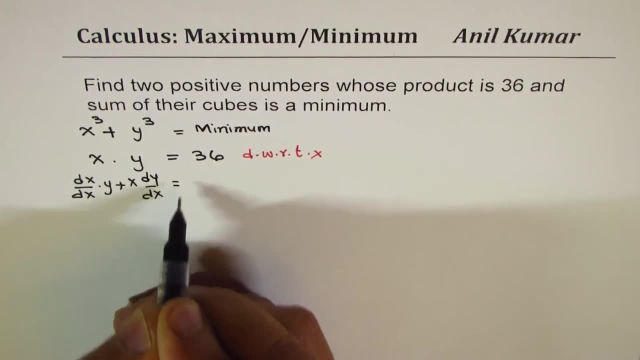 rule. So we have dx over dx times y plus x times dy dx, correct equals to d dx of 36.. Now this is y, so we have y equals to y plus x. dy dx equals to 0,, since derivative of a constant is 0. Now we can rearrange and 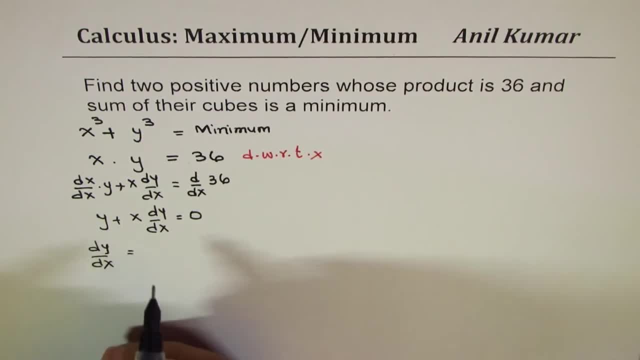 write dy dx in terms of x and y. So taking y on this side, we get minus y, then divide by x, So that becomes dy dx in terms of x and y. Now let us look into the first equation given to us. We want to minimize the sum of cubes, right? So we want to minimize the. 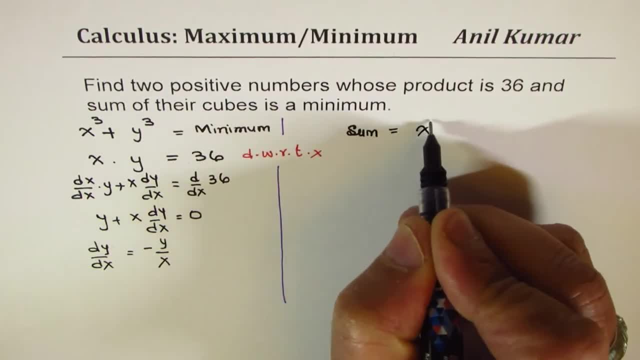 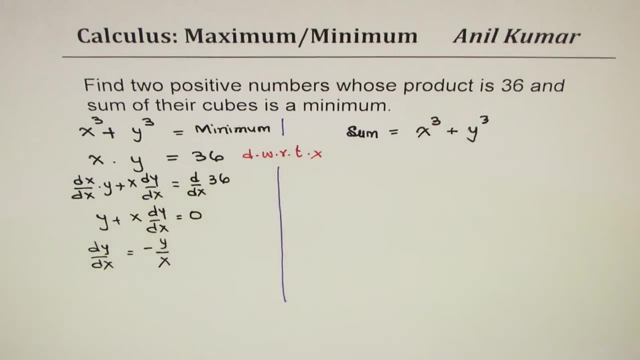 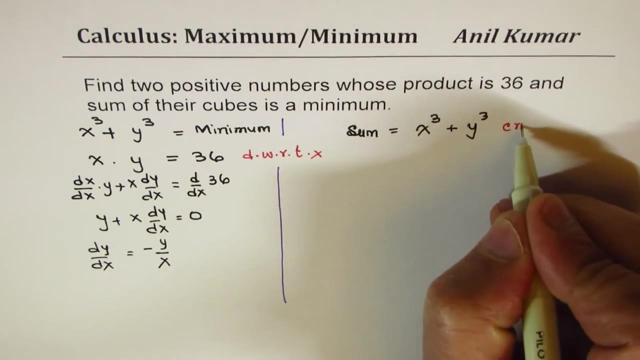 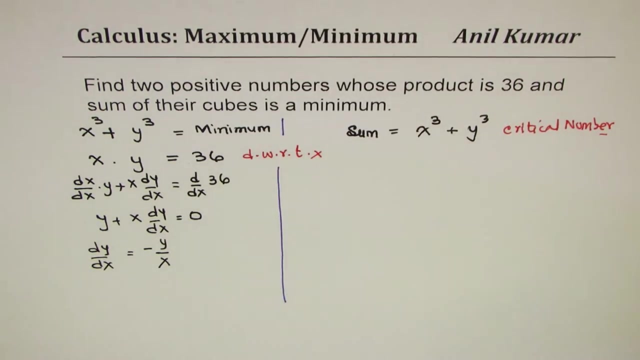 sum, Which is x cube plus y cube, right? So that means the derivative of this should be 0.. We will find a critical point here, So let us find a critical number. So again, differentiating with respect to x, let us call this variable as sum. okay, 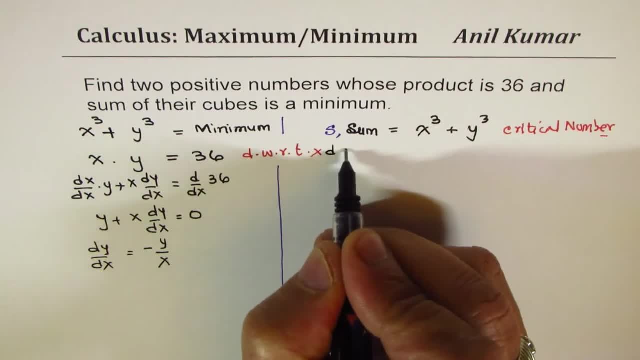 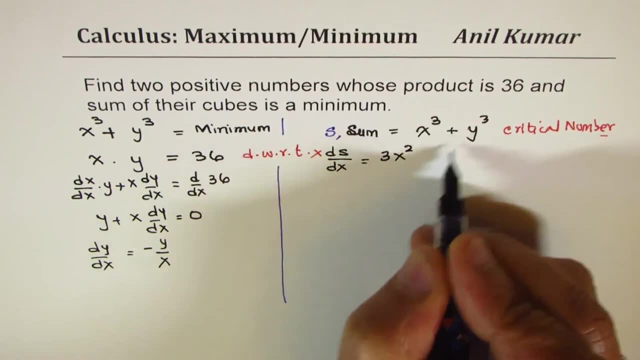 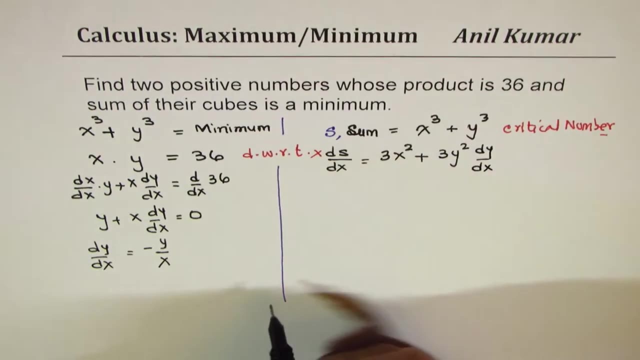 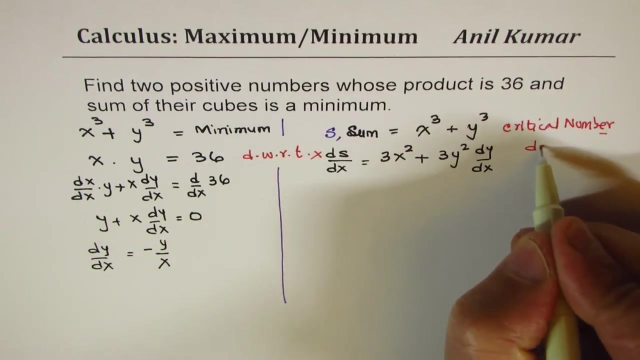 Then what do we get? We get ds over dx as equals to. when you take derivative, this becomes 3x squared. and here we get 3y squared, dy dx. Now for a critical number. this derivative should be 0, right, So we will equate ds dx to 0.. So the first derivative we are equating. 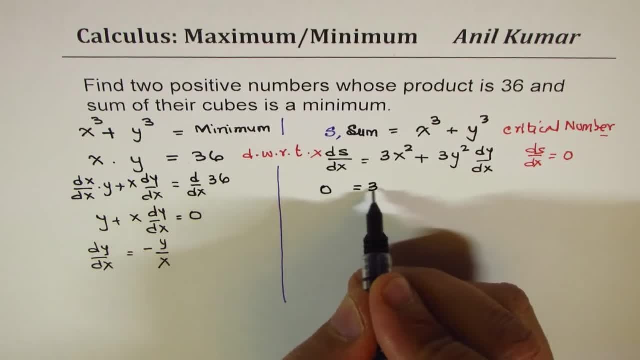 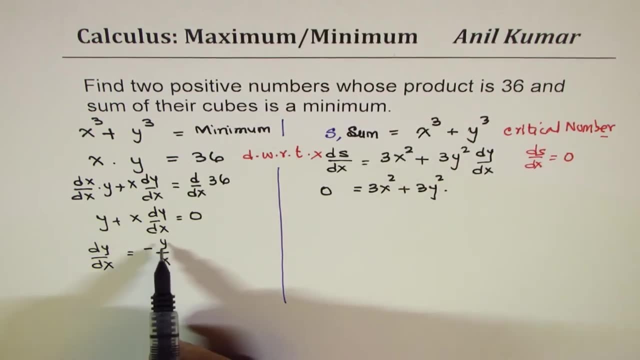 to 0, so we get 0 equals to 3x squared plus 3y squared and dy dx we just found as minus y over x, so we'll write this as minus y over x. so so that gives us. so minus makes this negative, so we have. 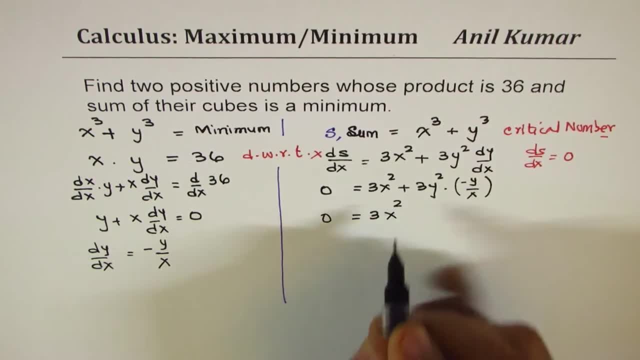 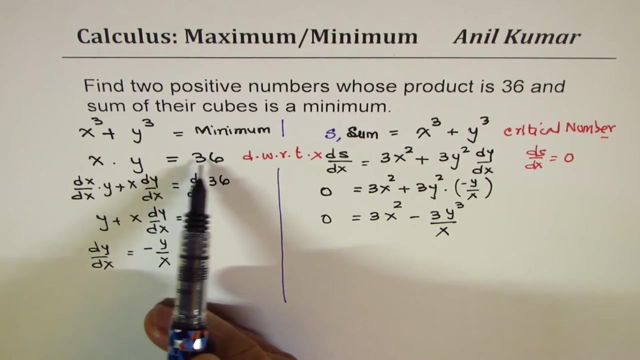 0 equals to 3x squared minus 3y cubed over over x. right, so over x. so that is what we get. now we need equation and only y, so we'll isolate y from here and we can write: y equals to 36 over x. so we also know y is equals to 36 over x. so from here we 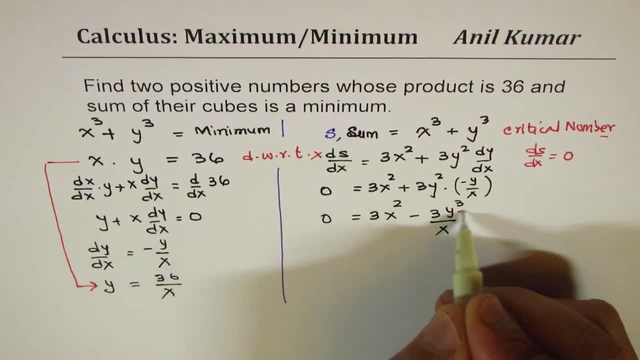 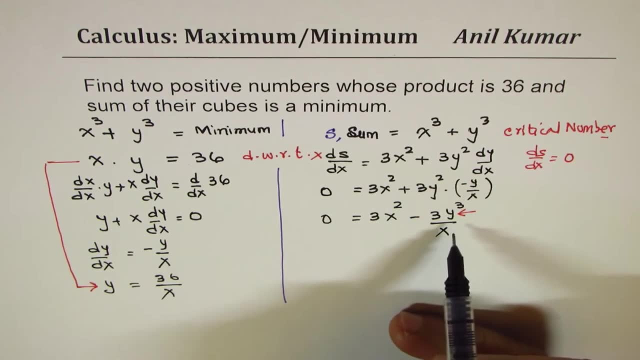 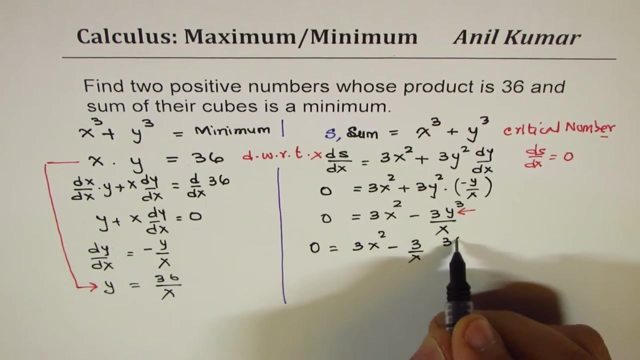 isolated y. we can substitute this y here. now you'll also notice that if I take- let me first change this right- so we'll write this as 3x squared minus 3, we'll change y to: so we have 3 here, 3 over x. let me write like this: and y cubed 36 over over x. 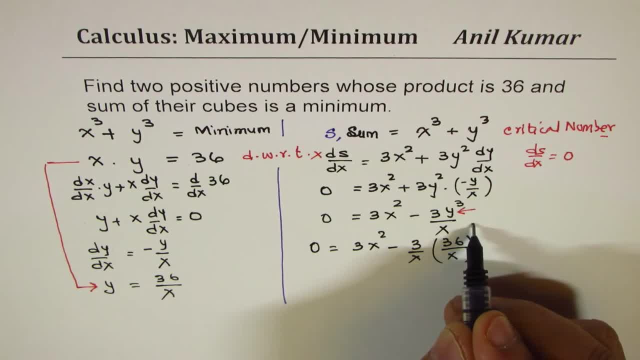 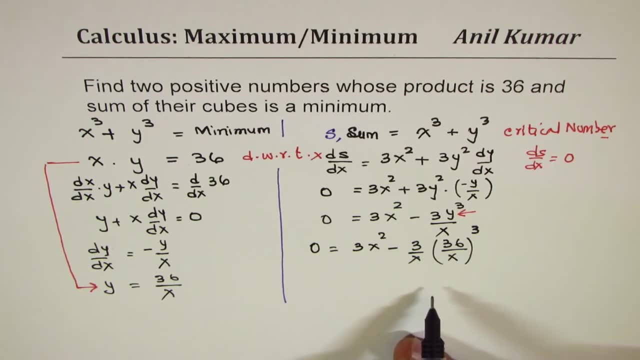 whole cube, that is y cubed right, 36 over 6 whole cube. so so we get that expression here. so 3 over x, that is over this. now to make this equal to 0, this is X to the power of 4 in the denominator right. so we can take 3: 3 is common over X to the power of 4, because 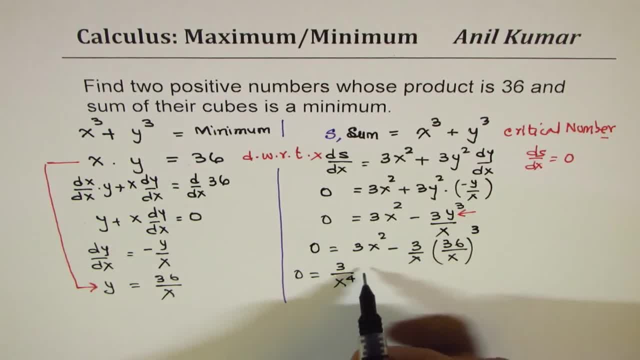 that is X cubed and this perfect. so what we get here is X to the power of 2 plus 4 gives us 6, right, and here we have 36 cube. so let me write this as minus 36 cube. okay, so that is what we get here. now for this expression to be 0. X to the. 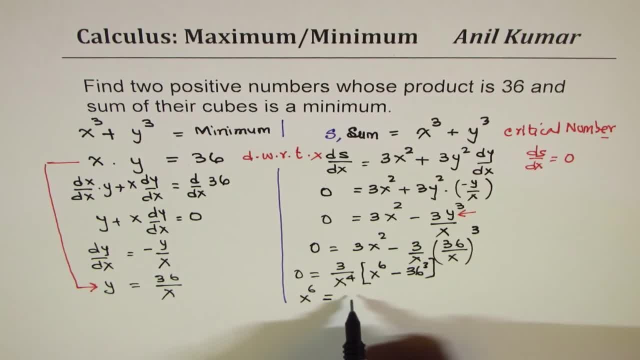 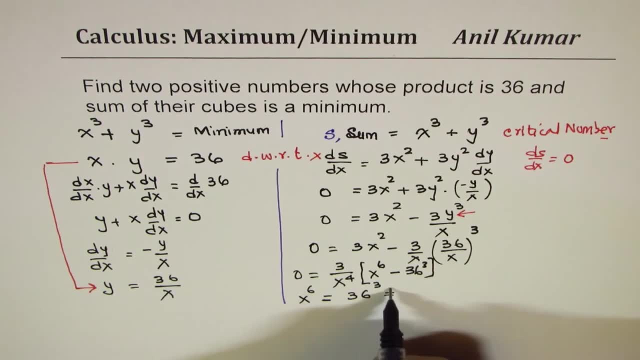 power of 6 should be equal to 36 cube, correct? Oh you are. this implies that X should be equals to 36, to the power of half great 6 divided by. I mean 3 divided by 6, which is half, and that gives you the answer as. 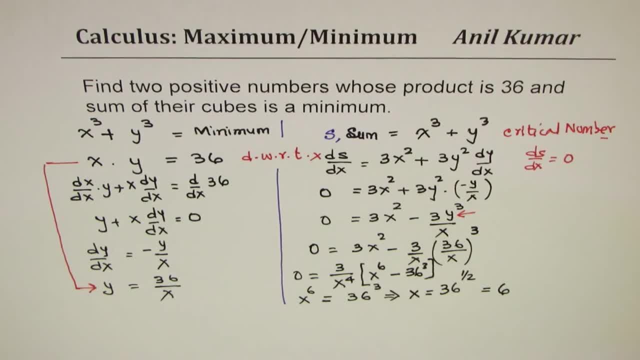 6. okay, so X is equals to 6. now, since X is 6, what should be Y? now, since X is 6, we can write 6 here. that is, 6 divided by 6 is also 6, right? so this is because we just found that X is equals to 6 and therefore Y is. 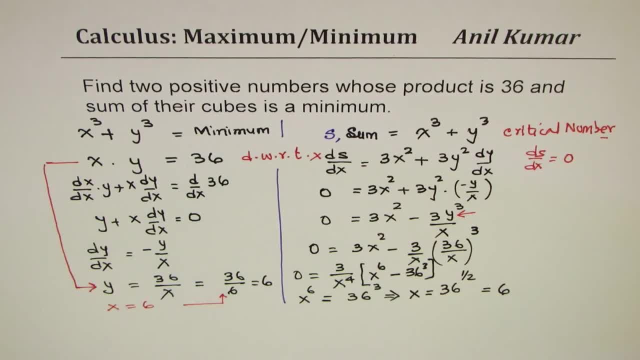 also 6. so find 2 positive numbers whose product is 36. in fact we got both as 6, so the numbers are 6 and and 6. now how do we say that it will result into a minimum? that's another important thing to understand. now, if I take derivative, 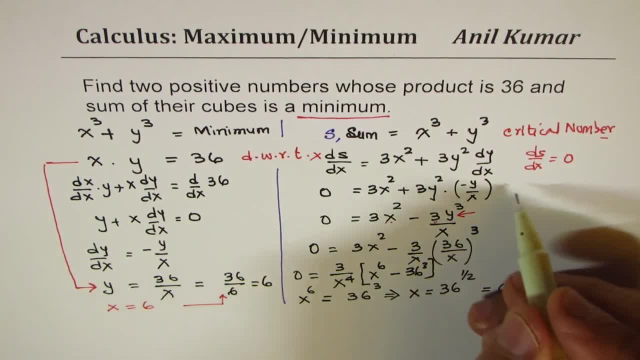 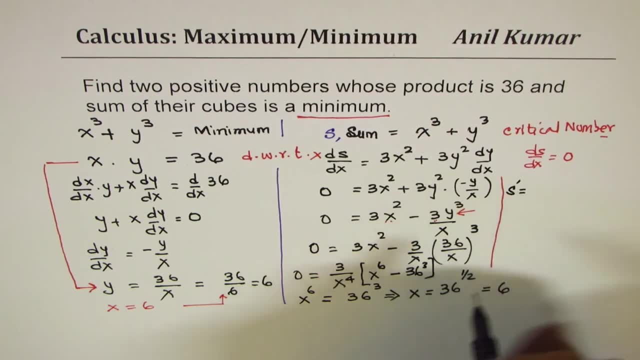 of this function here, or which may be written like this. let me just show you on the right side. so what we have here is that the first derivative of the sum is 3 x squared minus all this, which is a constant as 3 times 36 cube over X to the. 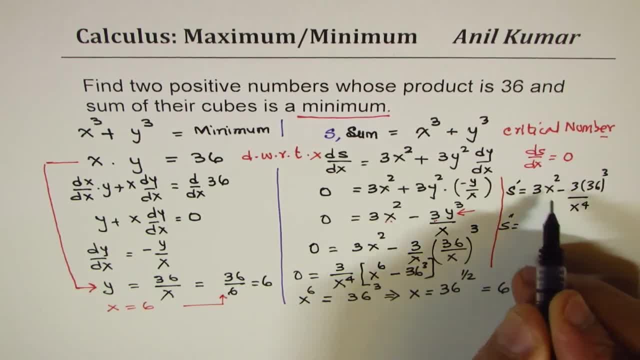 power of 4 right. second derivative for this function is going to be 6, X and that is in the denominator. so minus 4, that will make this as positive correct. positive 4 times 3 is 12 times 36 cube and minus 4 minus 1 will give me x to the power of 5 here. 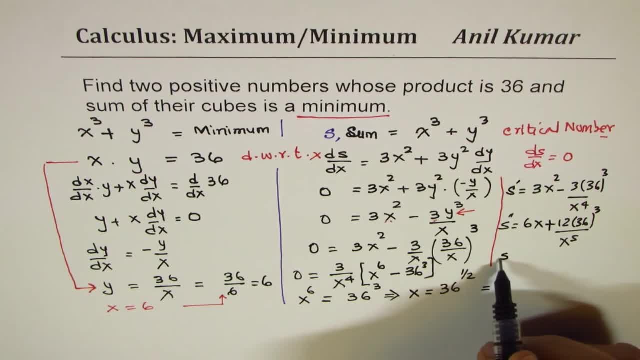 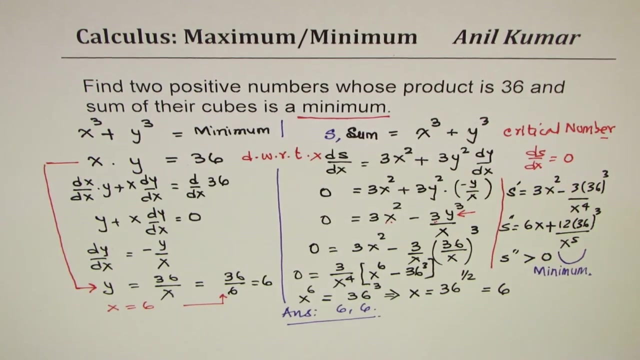 correct. so you know, this second derivative is actually greater than 0, right for any positive, two positive numbers, right. so this second derivative is greater than 0 and that means it's a concave upright and that means minimum, correct, and therefore our answer is that the numbers are 6 and 6, perfect. so that is how you.